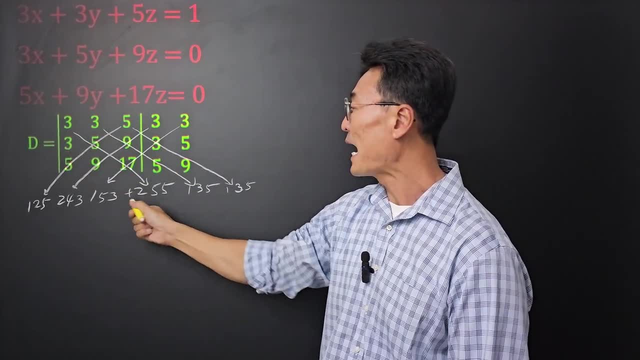 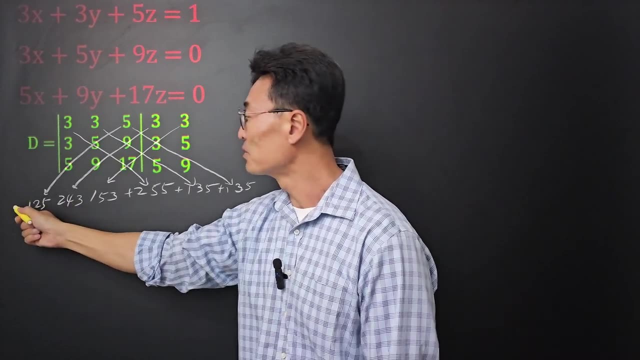 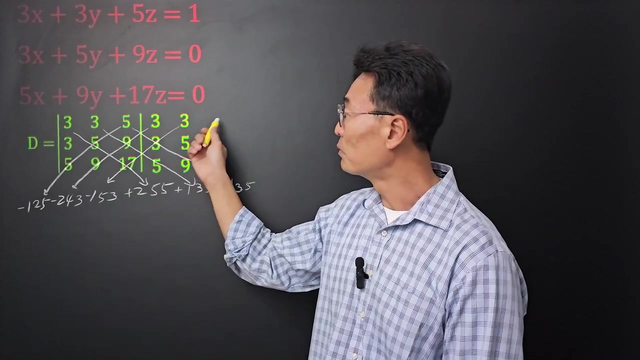 have from going from left and the right, we're going to be adding them, Whereas the product that we have from multiplying from right to left, we're going to be subtracting them. So, just as an example, if the product was negative going from right to left, 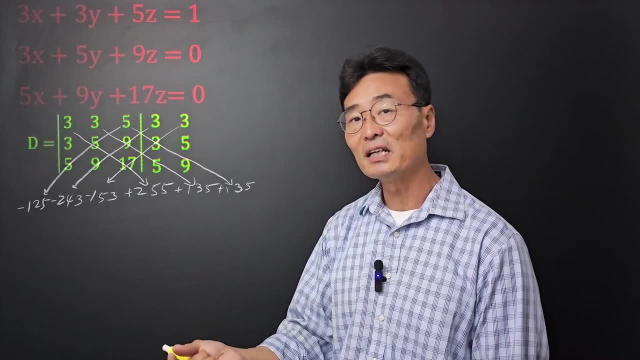 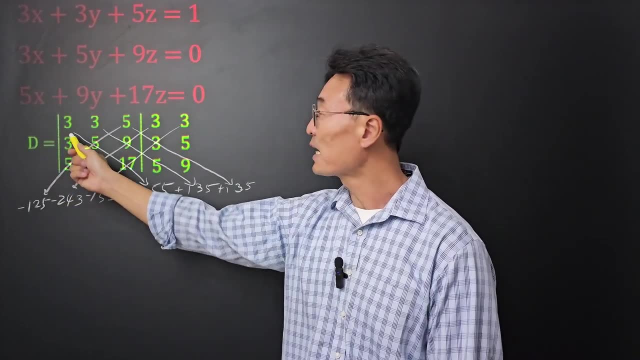 we're going to be subtracting the negative value, so it would have turned into positive, But, as you can see here all the products were positive. So any product that I have that I have from going from left to right are going to be positive, And then any product that I have from going from right to left. 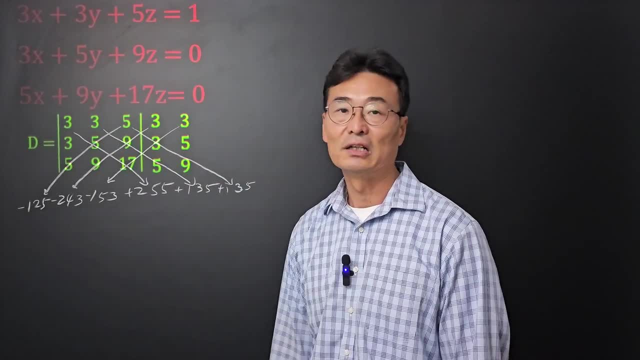 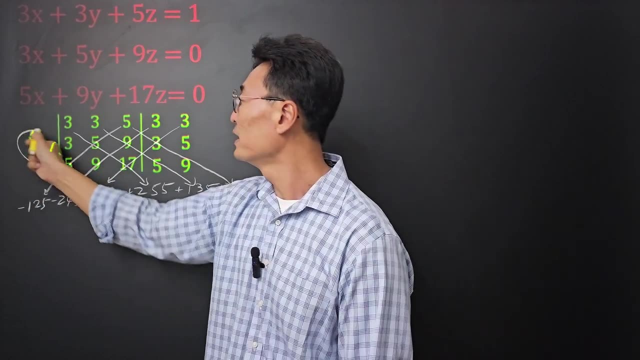 which were positive again, we need to go ahead and subtract them so they turn negative. So then, if I combine all this, we get a value of d equals to 4, since this whole thing is equal to d again, which is the determinant of the coefficient. 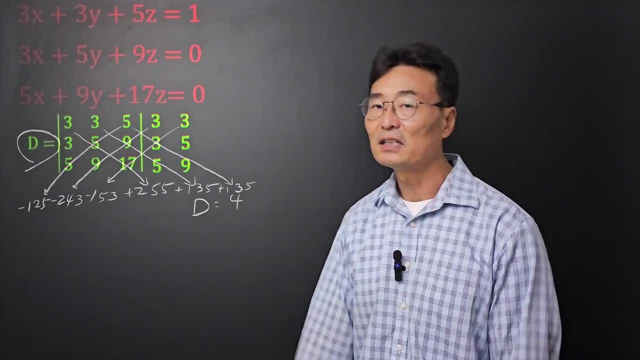 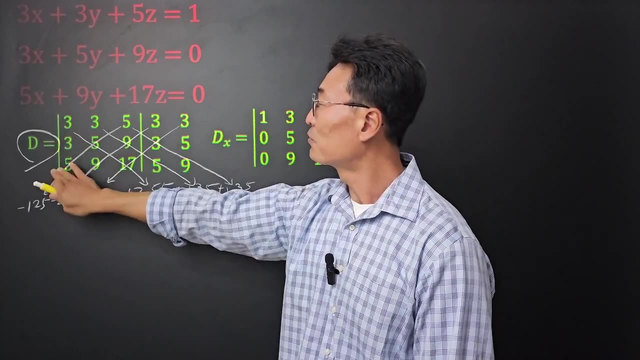 Of the variables that we have. Next, we need to find the value of d x. d x is going to be similar to what we did. Only difference is that the values that we have from the first column, the 3,, 3,. 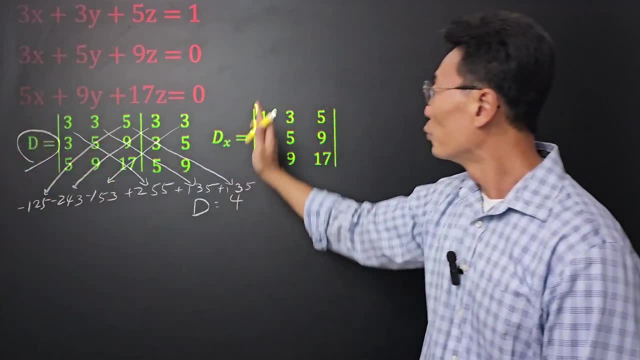 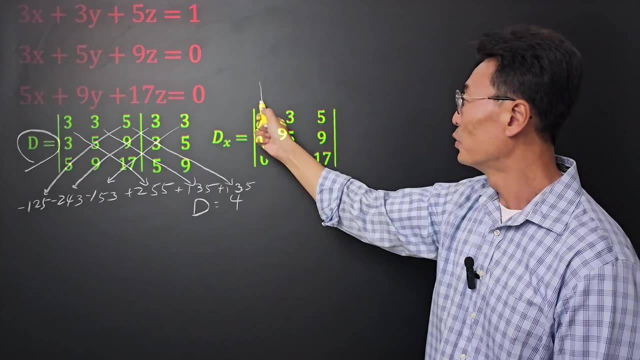 and the 5, or the 3x, 3x and 5x. we remove them and replace them with the numbers on the right side of the equal sign: the 1,, 0,, 0.. So notice: the first column is the only one that's changed. 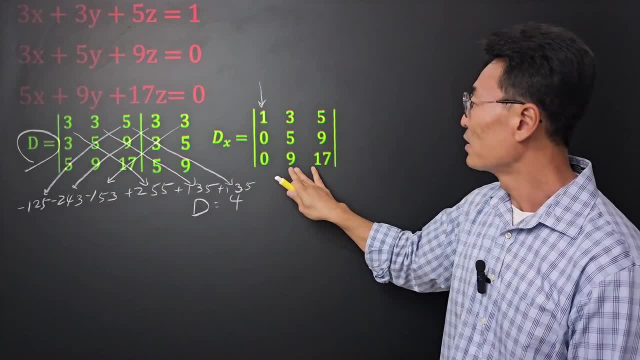 The second, which is a 3,, 5, 9, and the third, which is a 1, 0, 0.. So the first column is the only one changed, The second, which is a 3,, 5, 9, and the third, which is a 1, 0, 0.. So the first column is the. 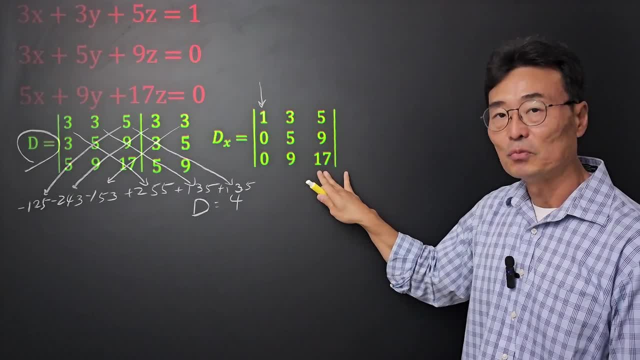 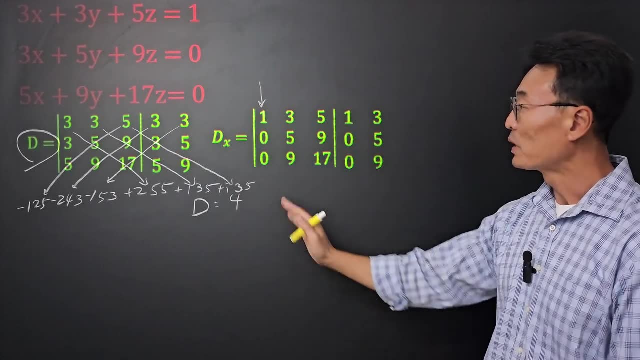 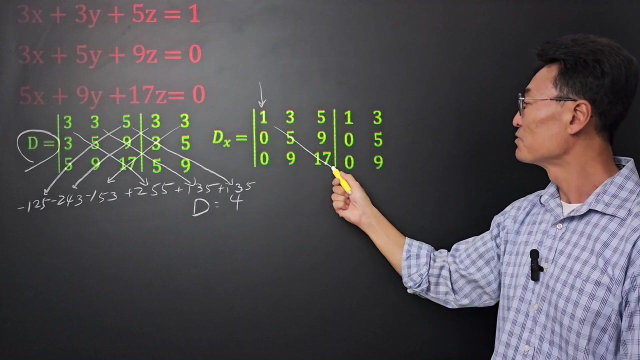 5,, 9, and 17 stay the same. Once again, we need to find the determinant of this matrix. We're going to be using the same shortcut method, meaning write down the first column and the second column on the right side and multiply So 1 times. 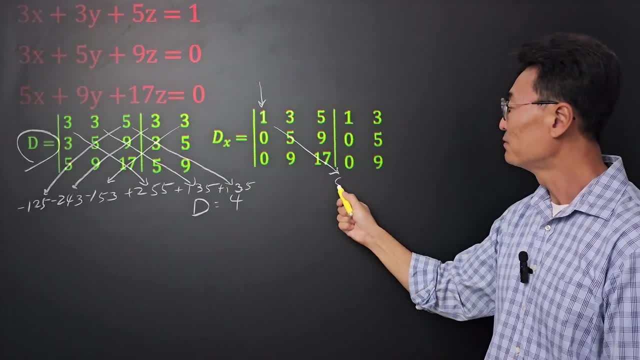 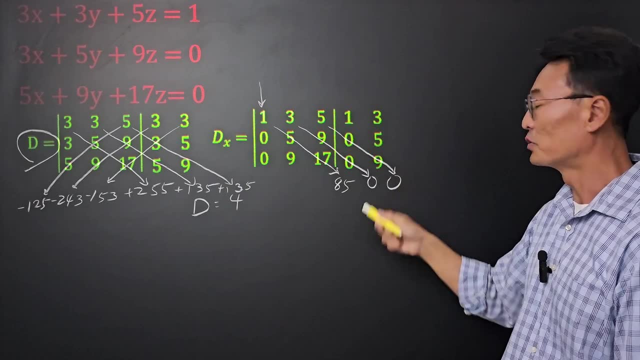 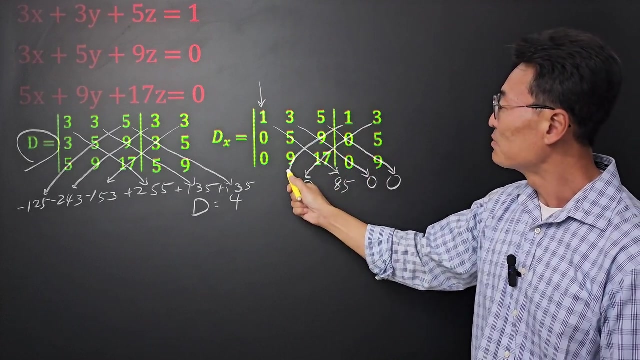 5 times 17 is going to be 85.. 3 times 9 times 0 is 0,, and 5 times 0 times 9 is 0 as well. Next, 3 times 0 times 17 is 0.. 1 times 9 times 9 is going to be 81,. and. 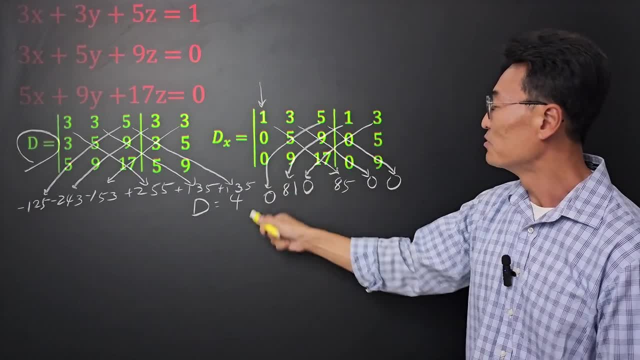 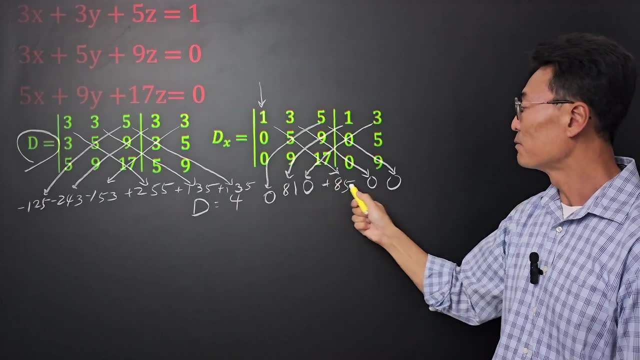 then 5 times 5 times 0 is going to be 0. But remember, anything that we have, or the products that we have, by multiplying from the left and the right, they get a positive value For, plus we add them, Any product that we have from multiplying. 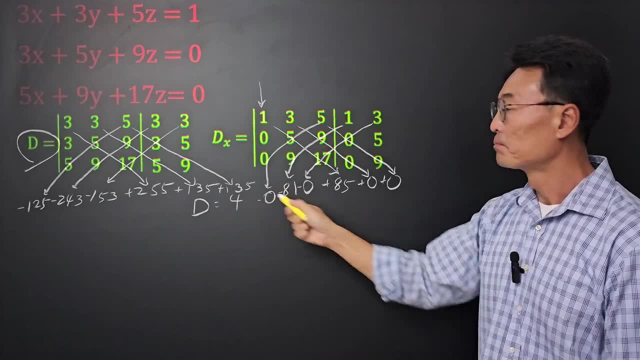 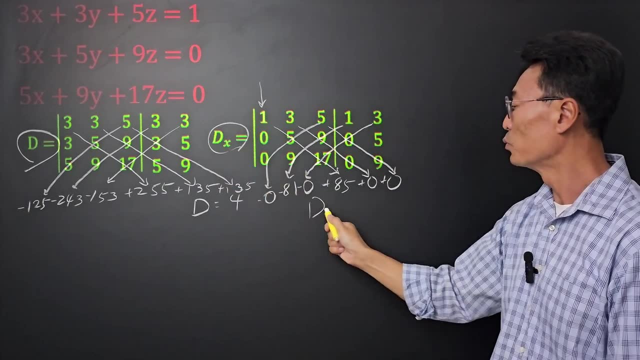 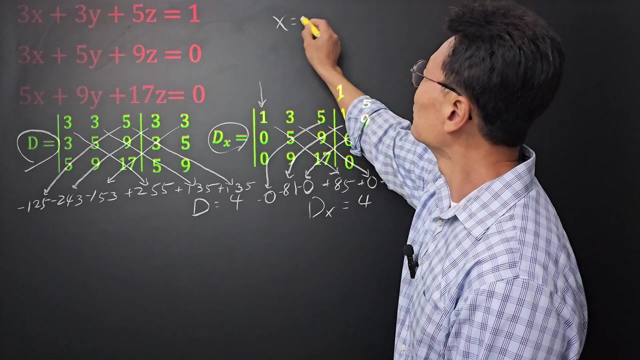 from right to the left. we subtract them. Luckily we have a bunch of zeros. makes our life easier. So if we simplify all this, the dx that we want is going to be positive four. Then to find x, all we have to do is we have to do dx over d, That's. 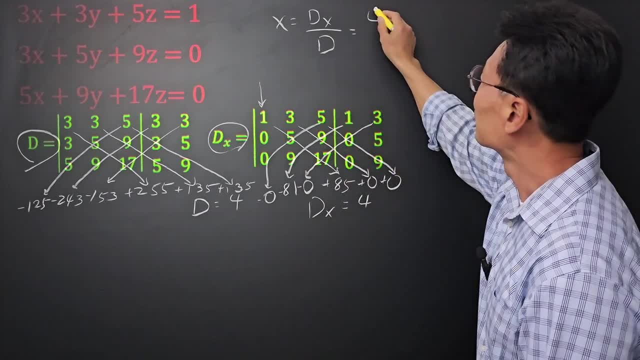 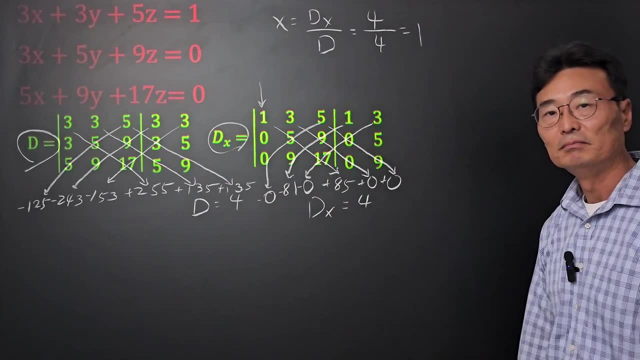 all we have to do. dx, we found, is four, So I'm going to put a four on the top, And then the d that we have earlier is going to be four as well. So the value of x is one. Let's continue with dy. 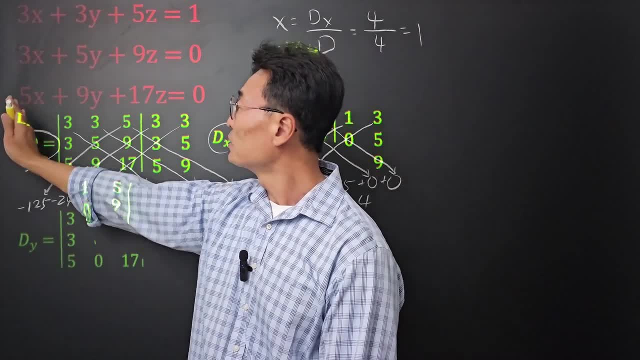 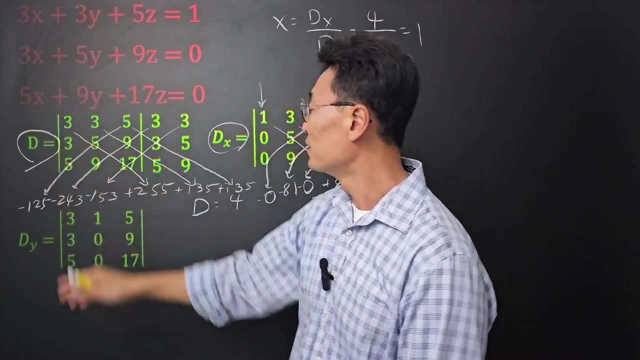 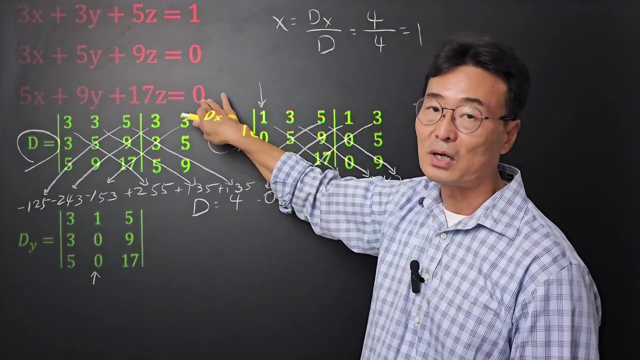 Dy. we leave the coefficients from the x alone, the three, three, five that we have, But the coefficients that we have from the y, the three, five and the nine, notice that we take it off and we replace it with the numbers on the right side of the equal sign, meaning one. 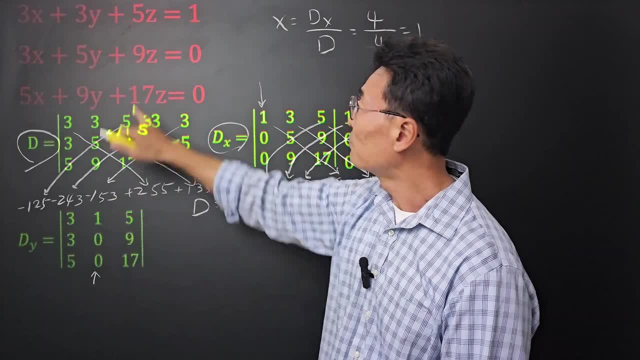 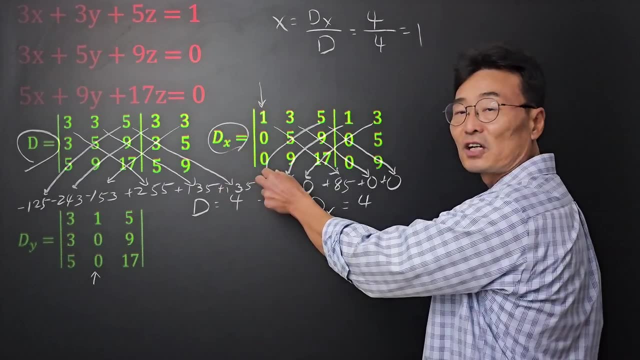 zero, zero, The coefficients of the z, the five, nine and the 17,. it stays the same. So, as you can see, when we're looking for the dx, we take off the first column or the coefficients of the x, replace it with the numbers or what the equation is equal to. 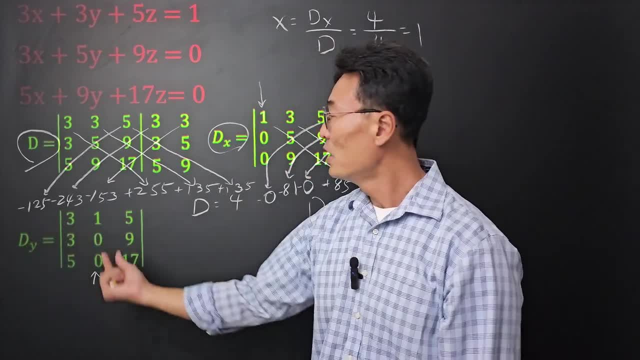 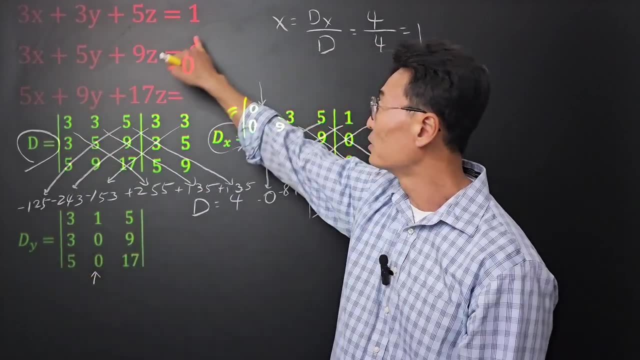 When we're looking for the dy, we leave everything alone. We take off the second column or the coefficients of the y for the dy. of course, we replace it with the numbers on the right side of the equal sign And, again using the same shortcut, I'm going to be rewriting the. 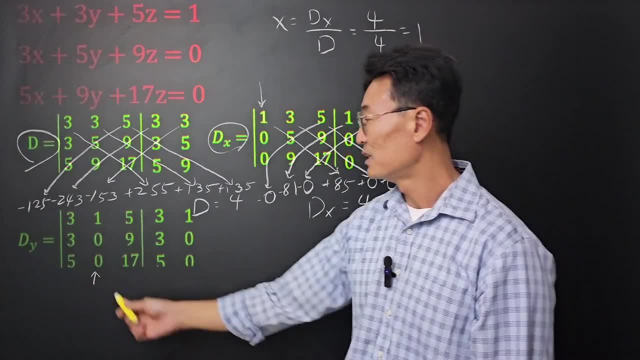 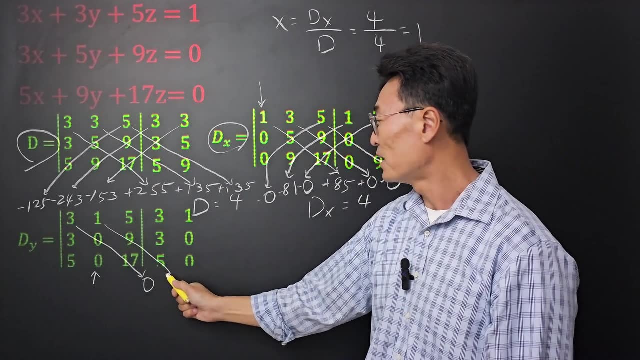 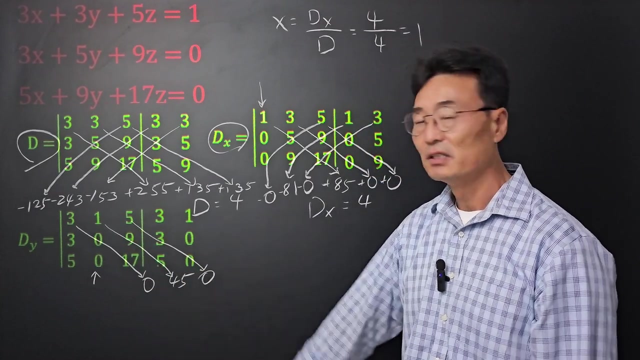 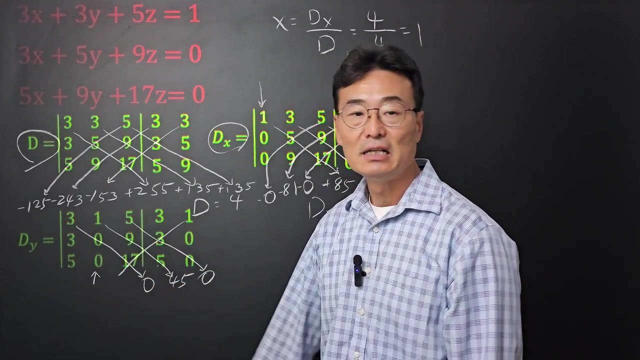 first column, second column, outside, like this: and then start multiplying Three times zero times 17 is 45.. One times nine times five is 45. And then five times three times zero is going to be zero. Next I'm going to go from right to left. One times three times 17 is going to be 51. 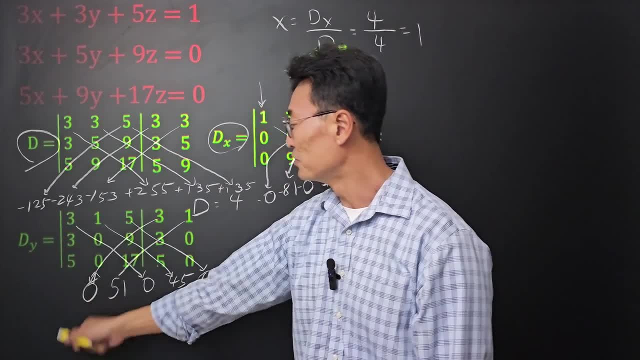 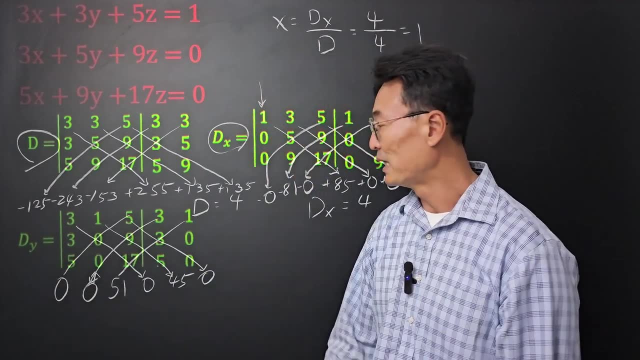 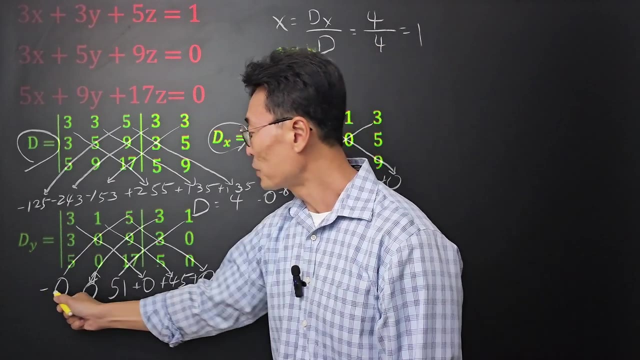 Three times nine times zero is going to be zero. And then, lastly, five times zero times five is going to be zero also, And we're going to be adding the numbers that we got multiplying left to the right. We're going to be subtracting the numbers we got by multiplying from right to left. 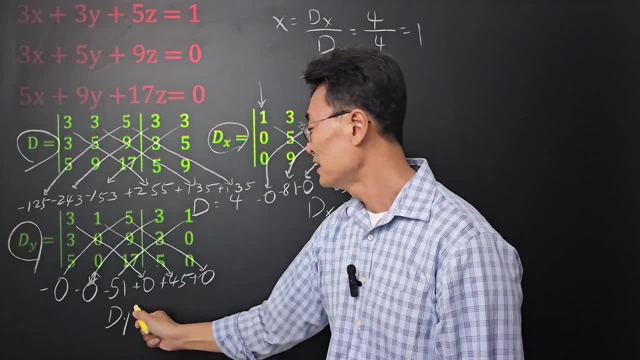 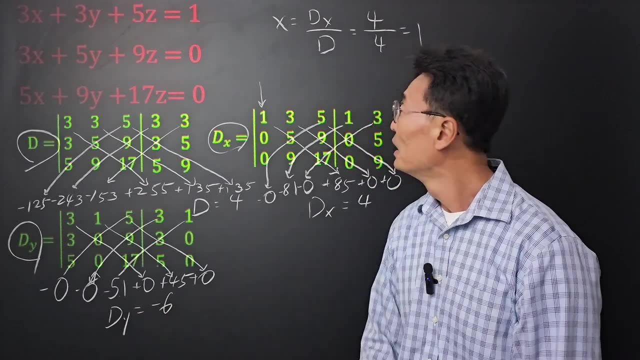 Then dy- since that's what we're solving for once again- is going to be negative 51 plus 45, or it's going to be negative six Here to find the value of y. we're going to be doing dy over. 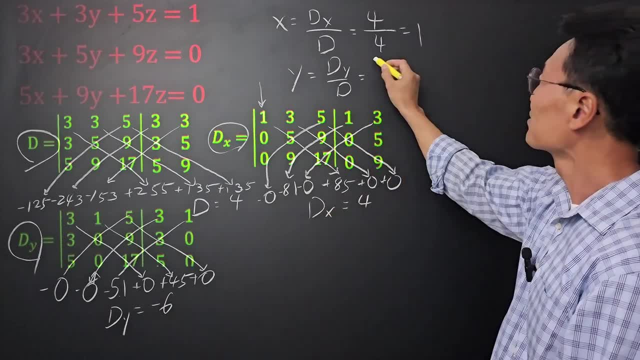 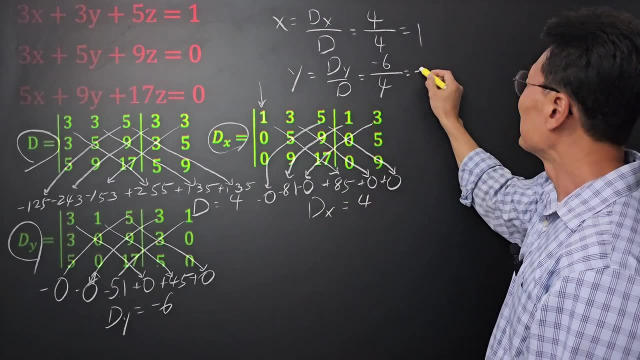 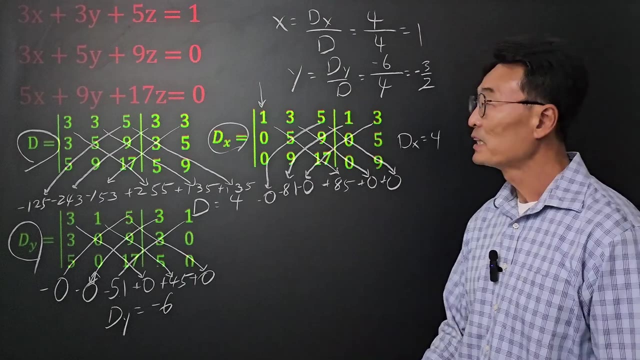 dy, where dy, we just found, is negative 6, and then d, of course, is 4, and now all you have to do is reduce this and we get a negative 3 over 2 for the value of y. So at this point, now that we know the value of x and y, we could play into one of the 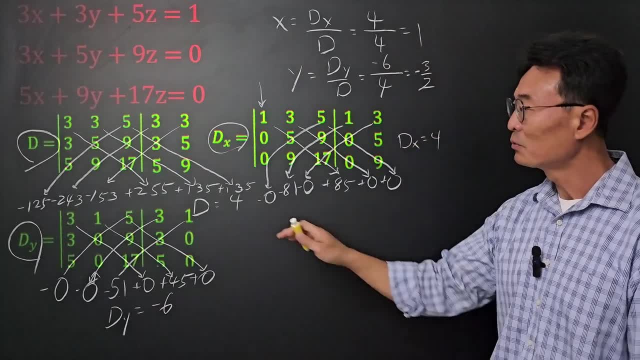 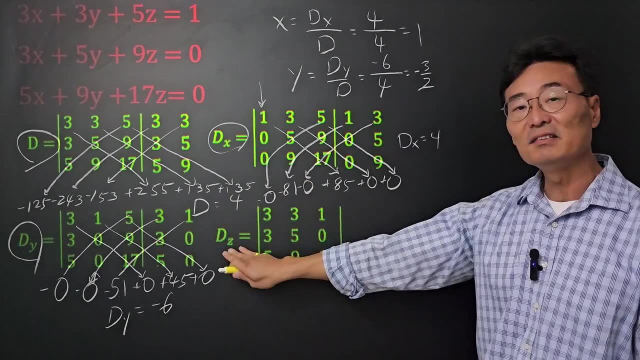 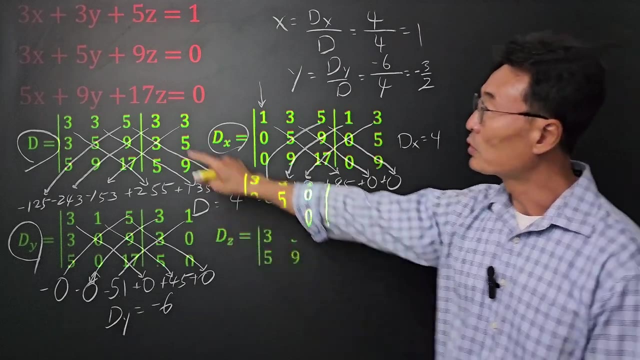 equations and find the value of z. but I want to repeat the process to give you the actual practice on how to find the determinants. So, to find dz, we leave the first and the second column alone and we replace the third column, or the coefficients of the z, with the numbers on the right side of the equal sign: 1, 0. 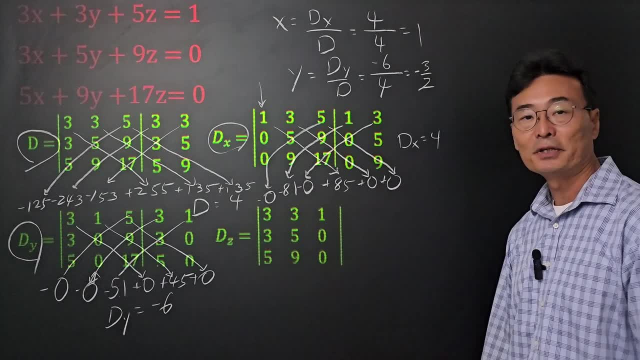 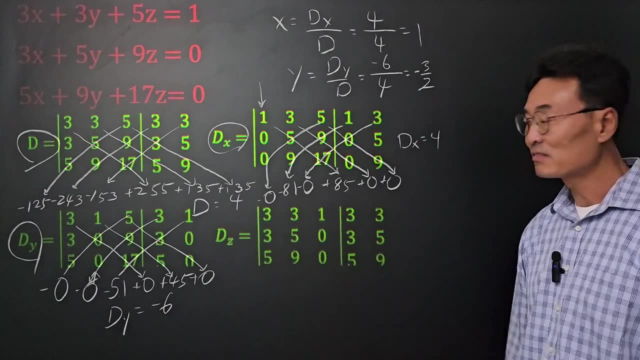 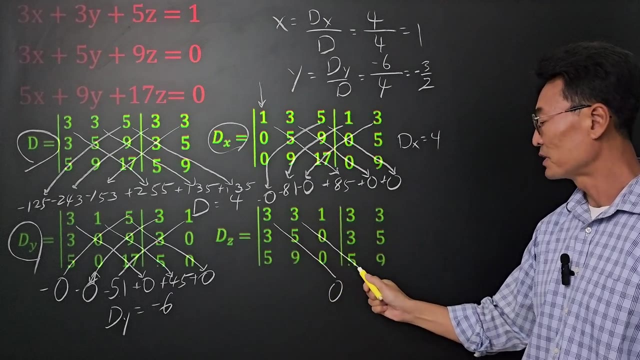 0.. Then again, to find the determinant of this 3 by 3 matrix, we're going to be using the shortcut, Rewrite the first and the second column on the right side, and that's right. We're going to multiply again. 3 times 5 times 0 is 0.. 3 times 0 times 5 is 0, and 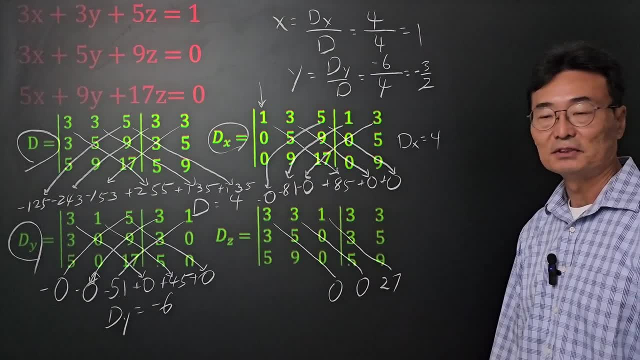 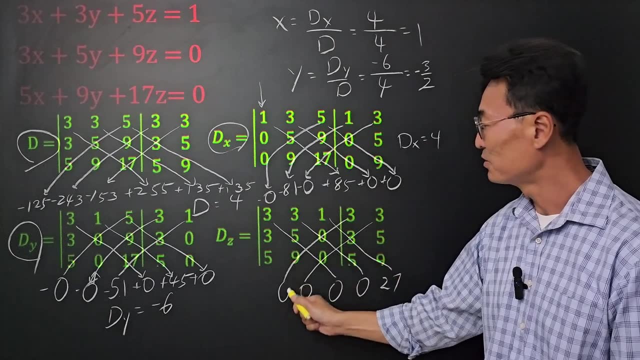 1 times 3 times 9, of course, is 27.. And then I'm going to go from right to left. 3 times 3 times 0 is 0.. 3 times 0 times 9 is 0, and 1 times 5 times 5 is 25.. We. 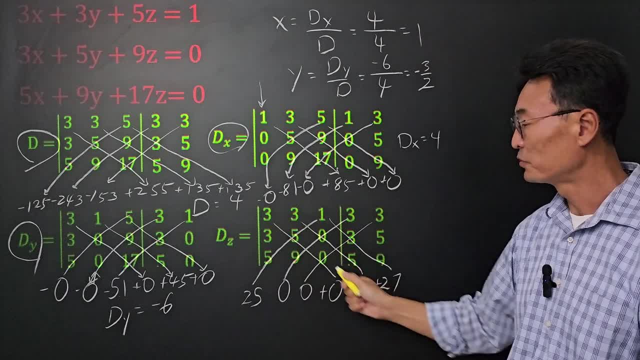 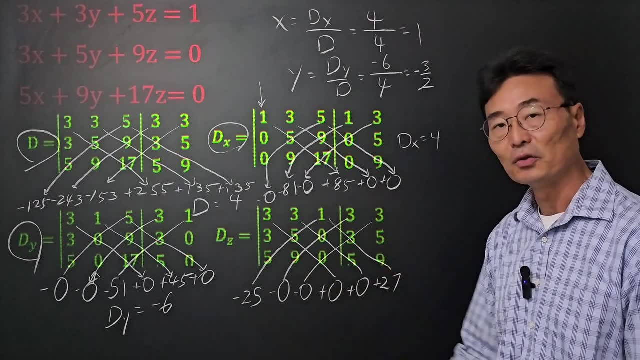 add the products that we got by multiplying from left to right. However, we're going to be subtracting the numbers that we got or the products that we got by multiplying from right to left. So if I combine all this and we get dz is. 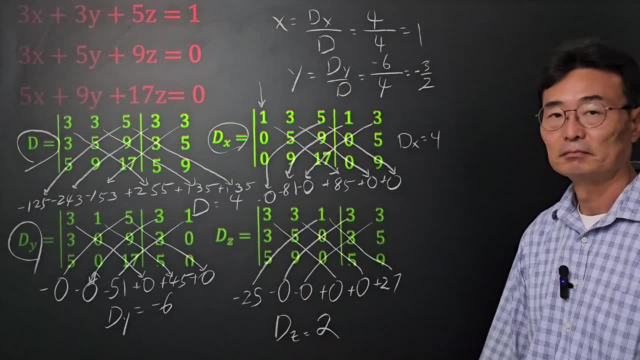 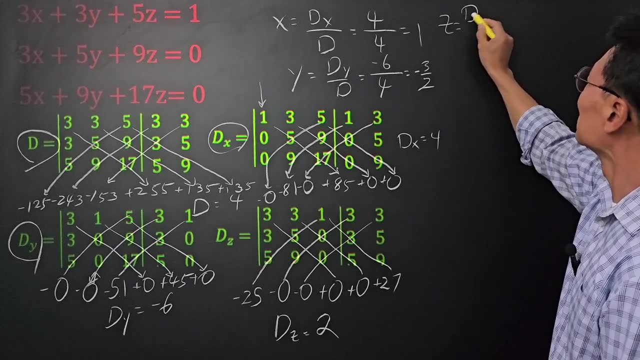 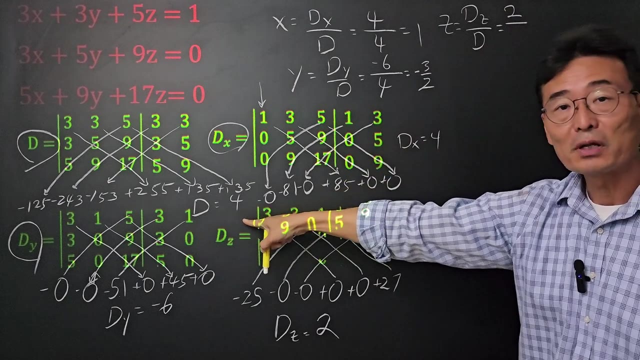 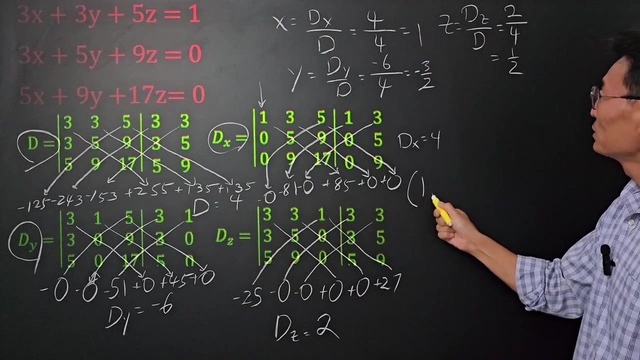 going to be positive, 2.. So then, our final answer for z is going to be dz over d, where dz is 2, and d, of course, was 4 that we found earlier. So that's going to be 1 half, And our final answer is going to be 1 negative 3 over 2 and 1 half.